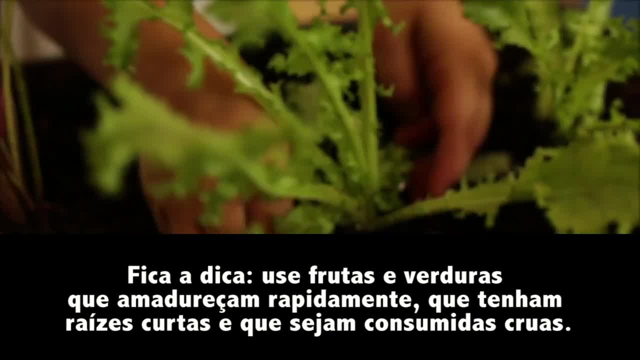 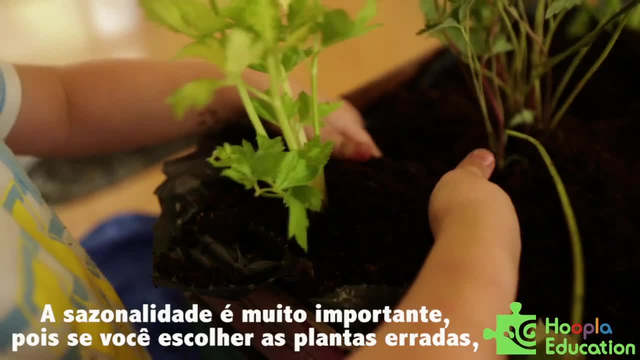 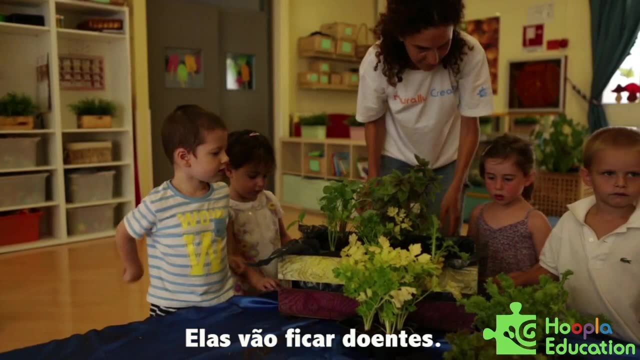 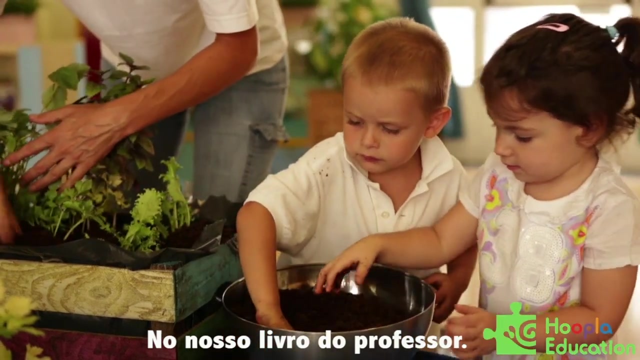 Seasonality is really, really, really important because if you choose the wrong plants, they won't grow, they will get sick. So before choosing the plants, check with our list in our teachers book and then otherwise you can also check online, but be sure you choose the right plants. 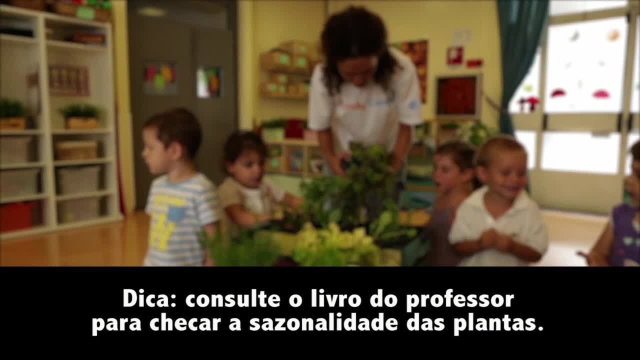 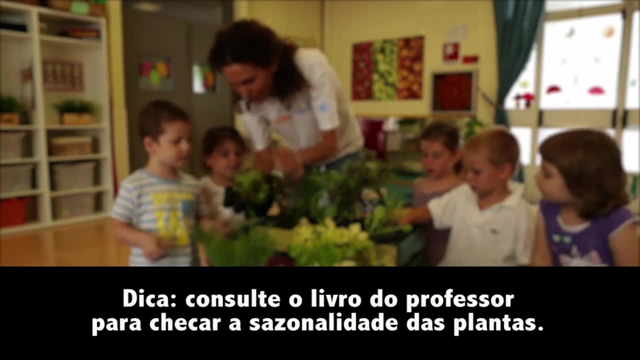 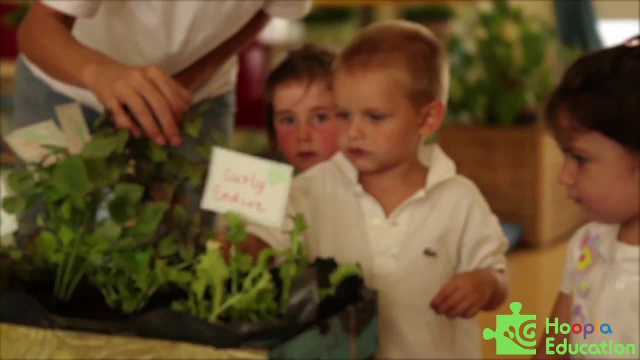 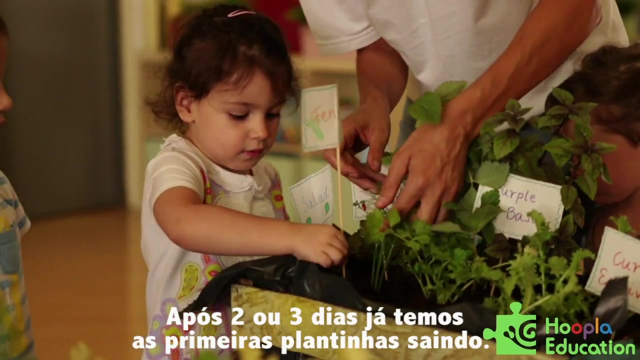 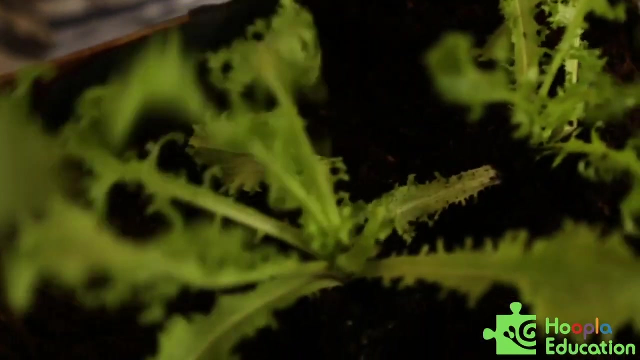 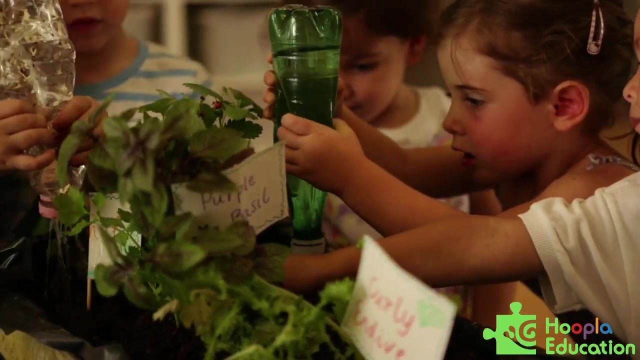 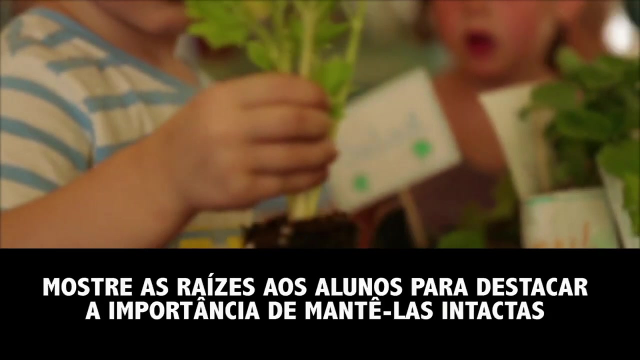 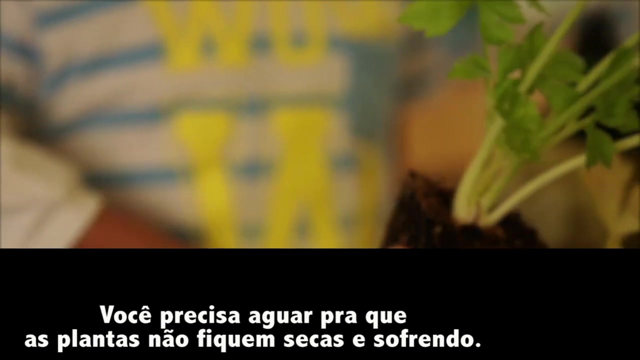 Salads grow quite quickly. after the first two or three days you will have the first small plants coming out, and after two or three weeks you can start collecting the first small leaves. You would need to keep it watered, of course. it shouldn't dry out because plants will suffer. 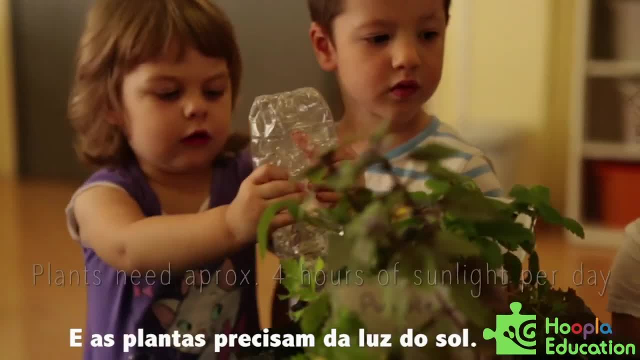 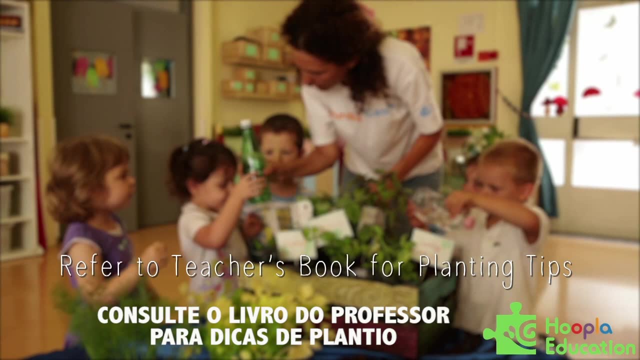 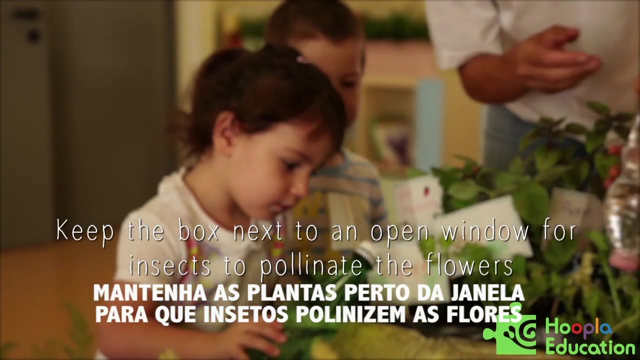 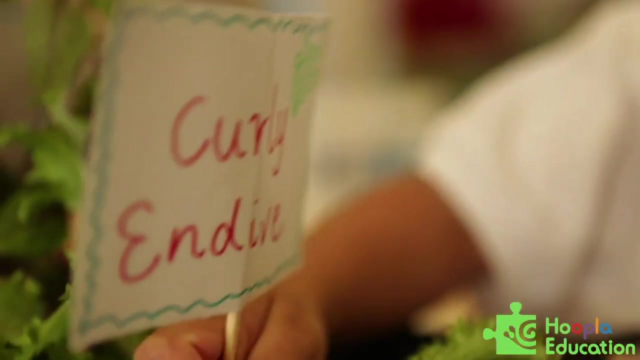 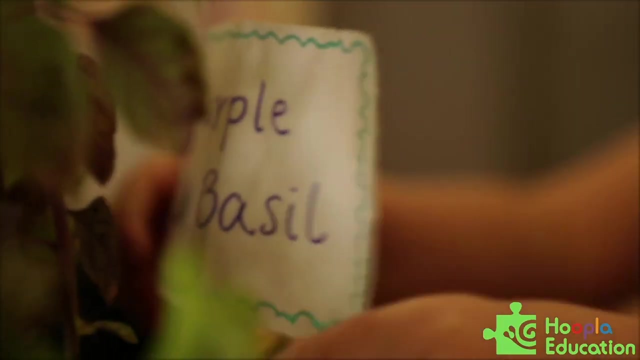 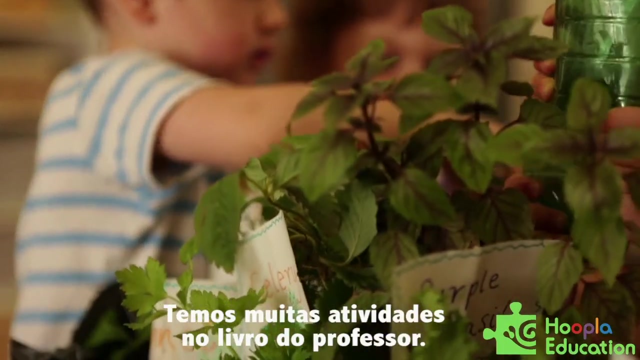 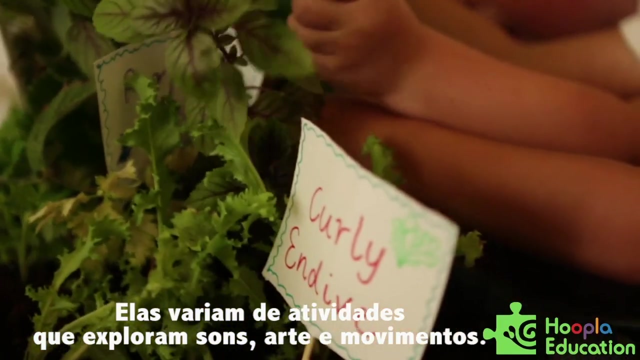 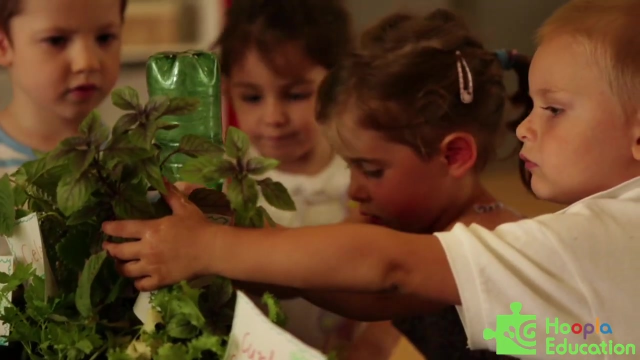 You have to be careful not to water it too much, And then plants need some sunlight. In the teachers book we have many, many activities that actually vary from sound, exploration, art activities, movement. We made this journal because we thought it would be nice for kids to have actually a 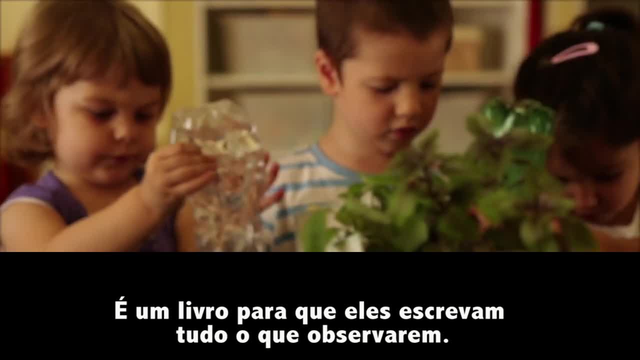 book where they can write everything, they everything, they see all the things that they see, all the changes and they can really monitor their plants and document everything.